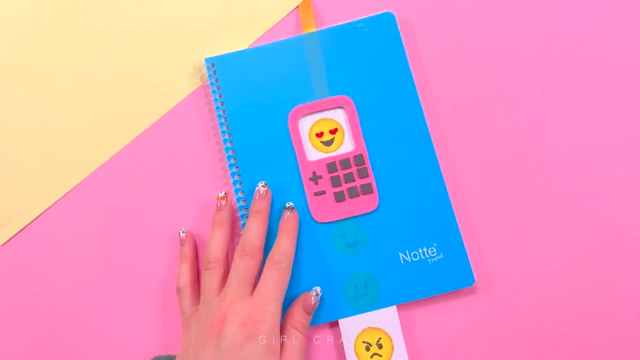 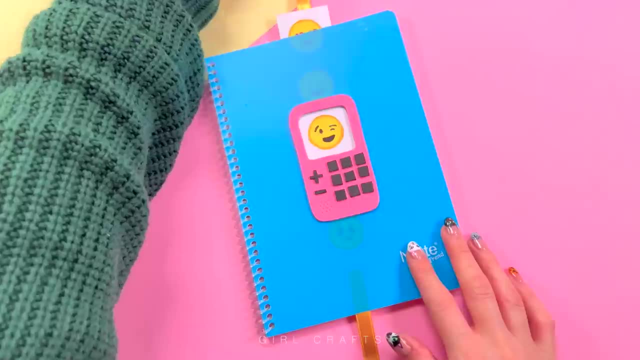 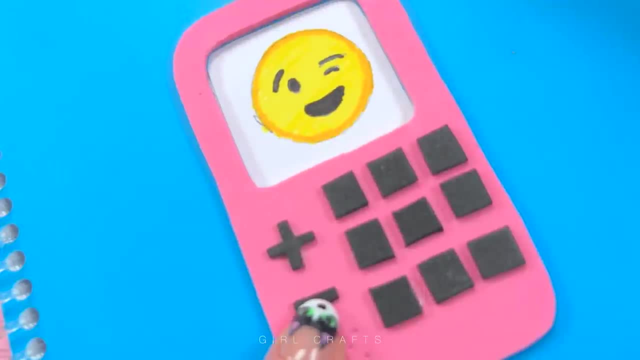 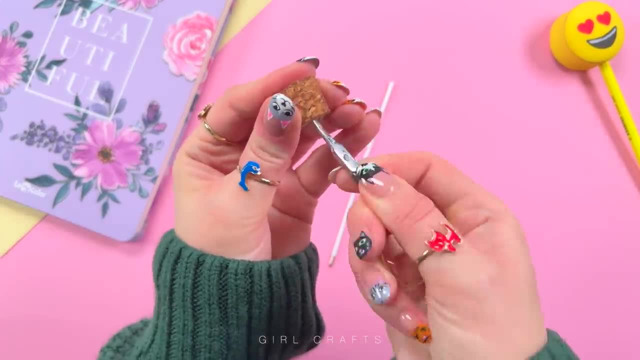 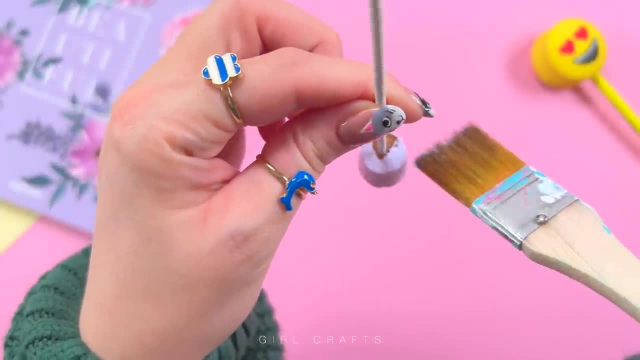 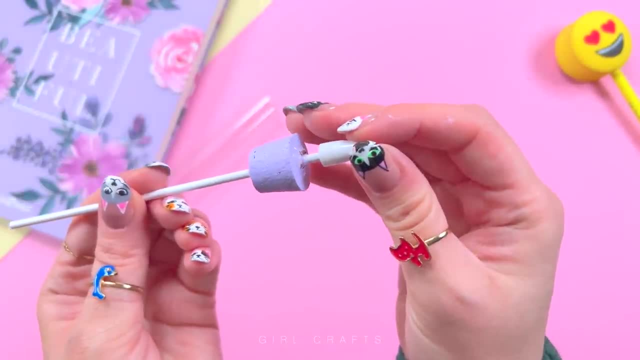 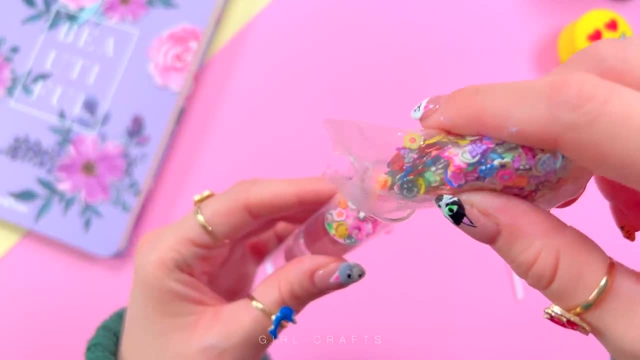 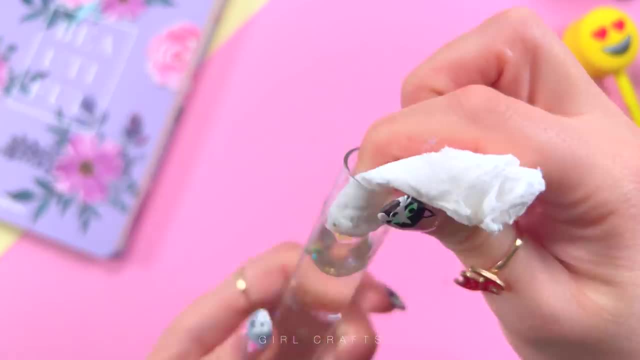 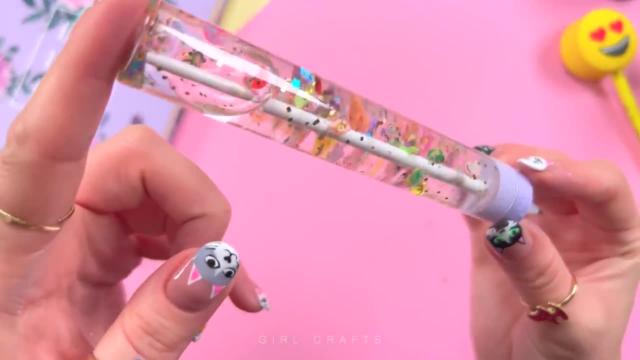 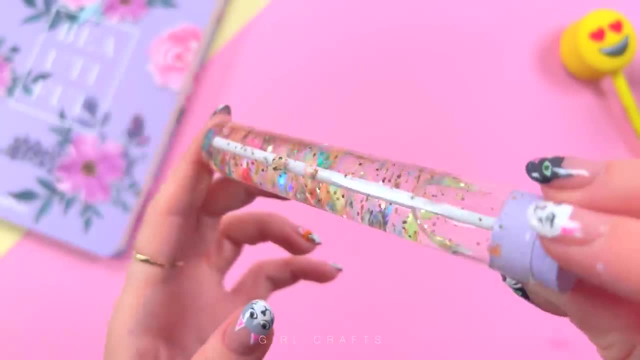 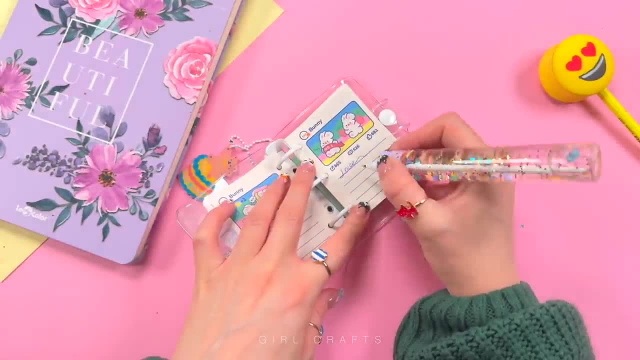 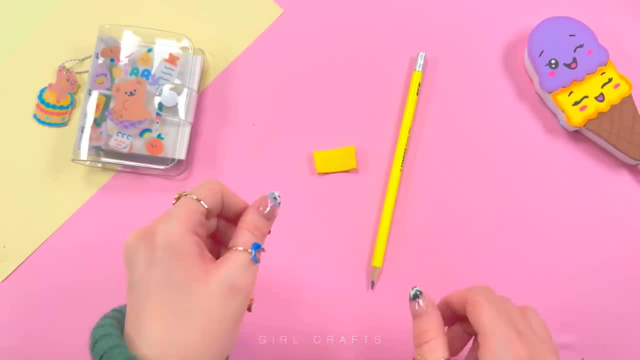 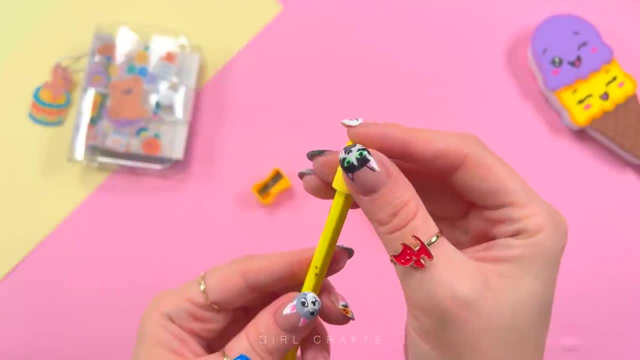 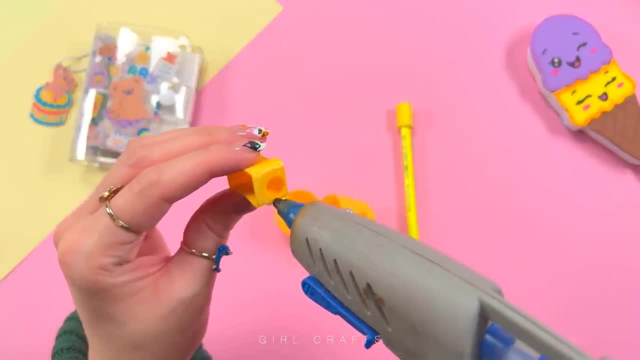 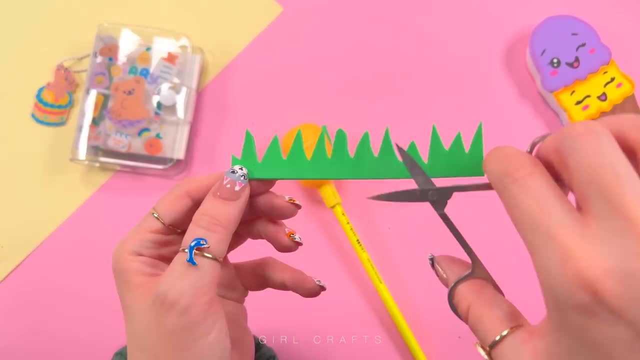 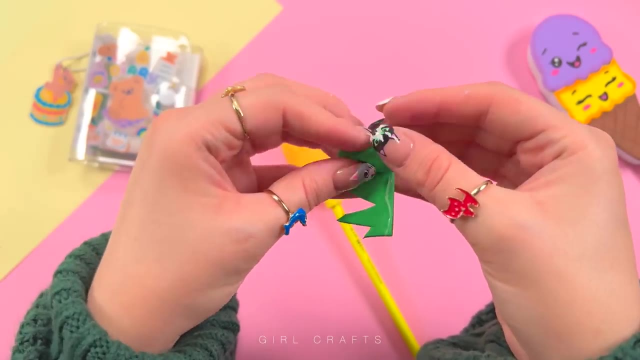 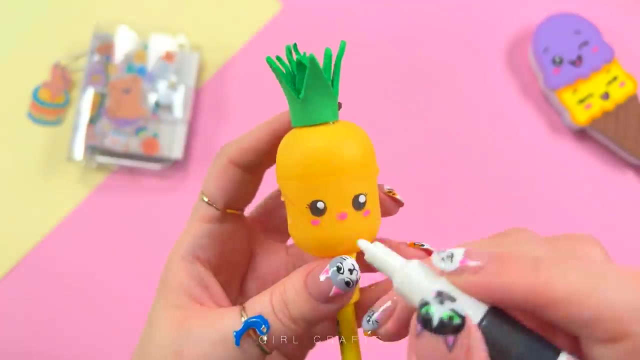 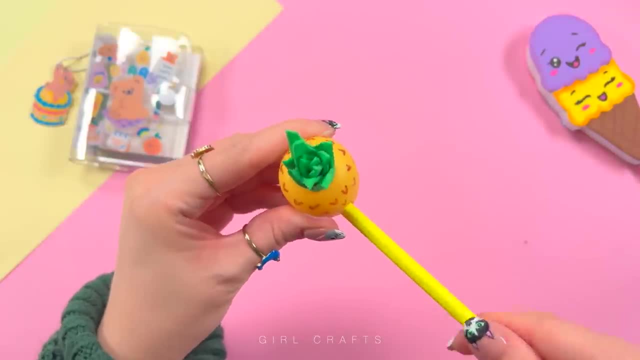 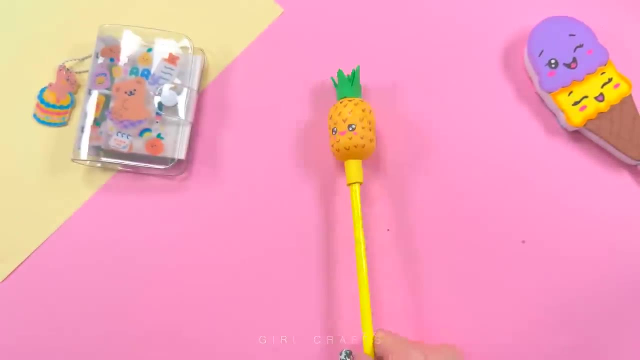 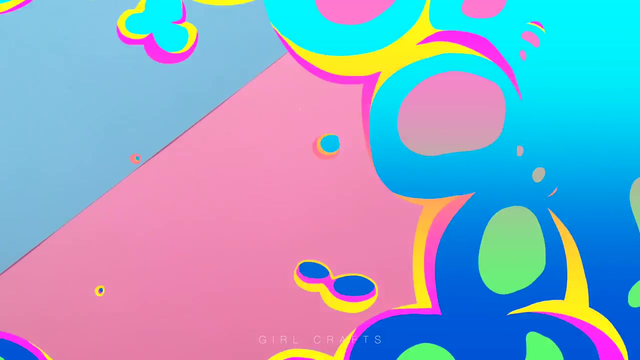 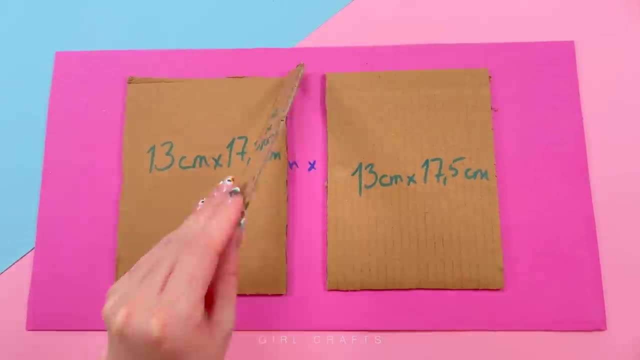 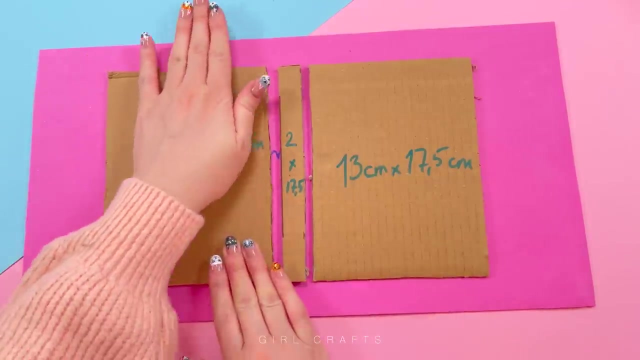 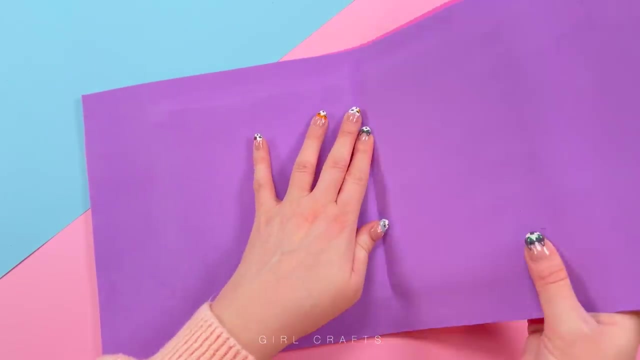 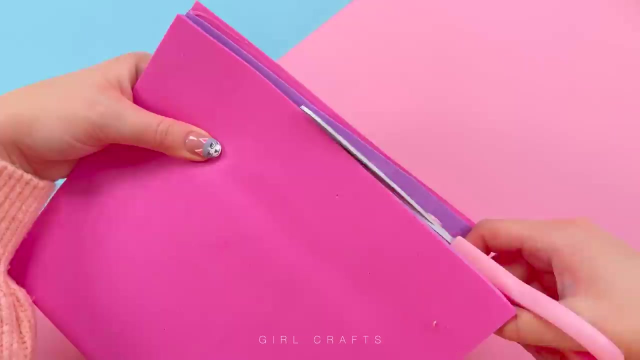 The stars are shining brightly up above me. It's beautiful, this world, And the firefighters dance in circles all around me. Oh, oh, oh, oh. Let's shout it out. Oh, oh, oh, it's beautiful, Oh, oh, oh. everything we see. 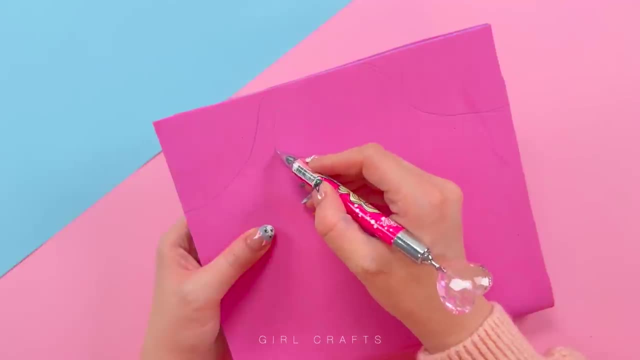 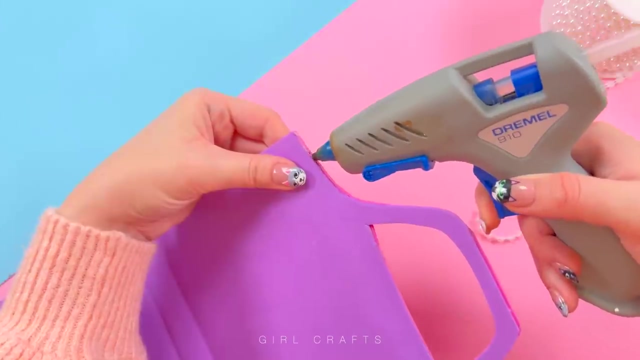 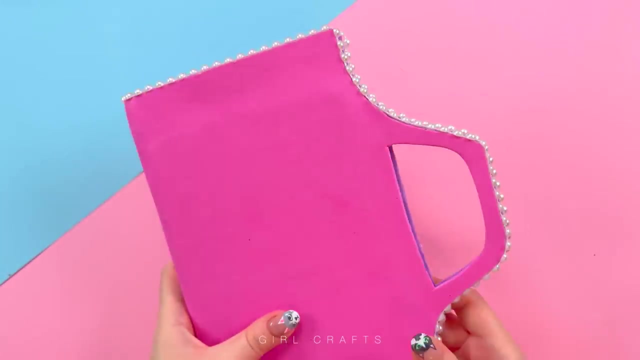 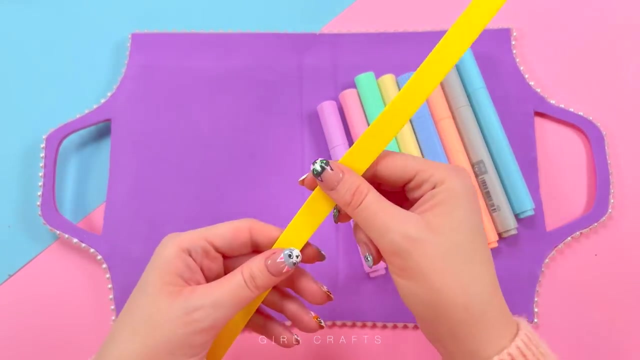 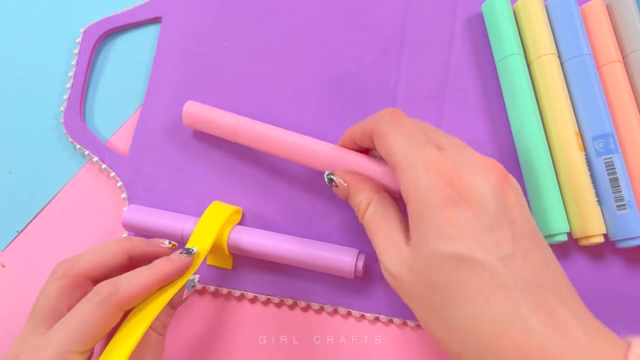 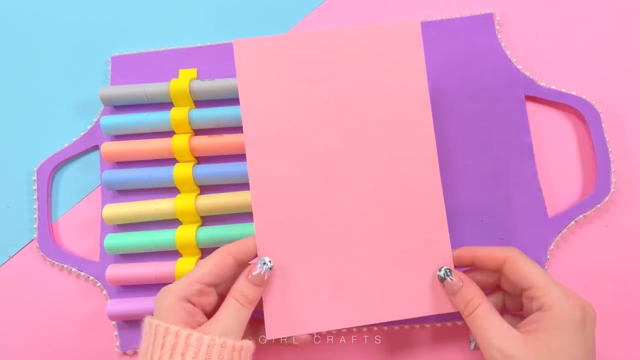 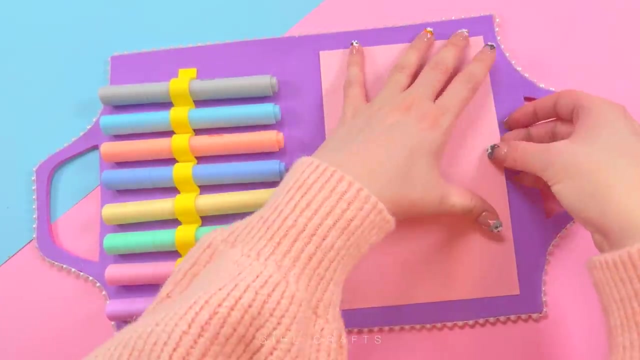 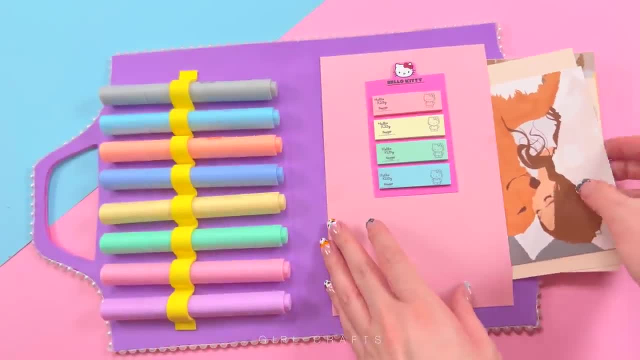 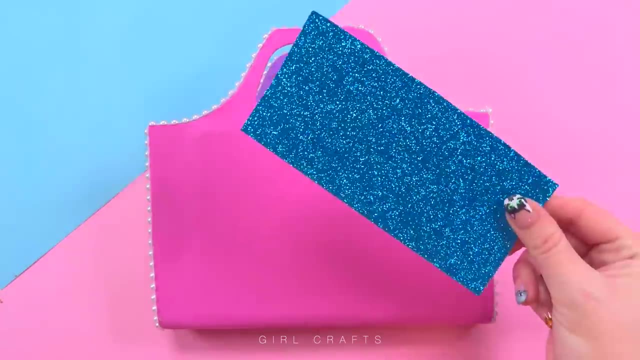 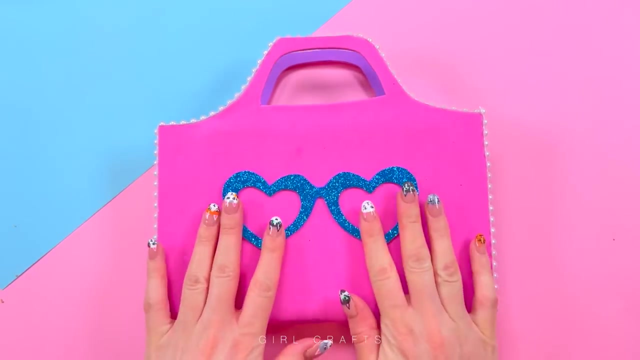 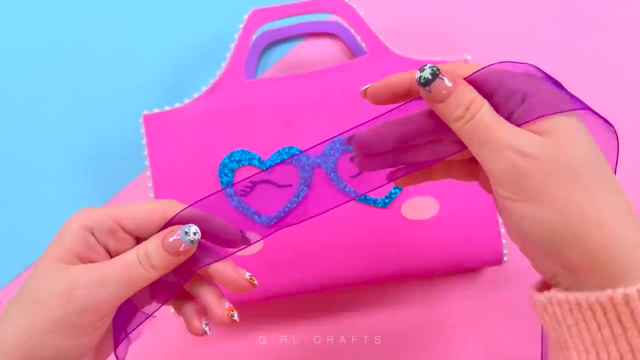 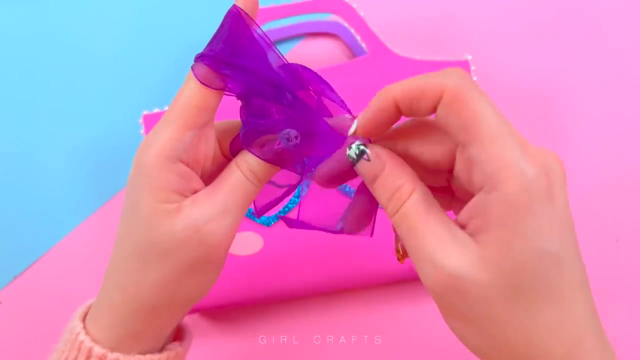 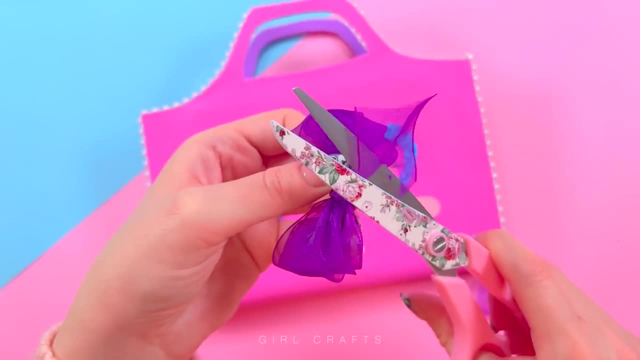 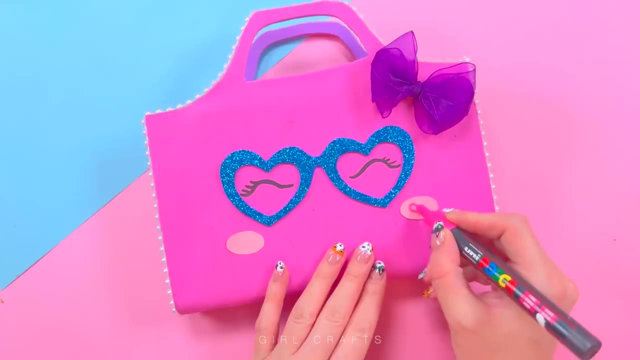 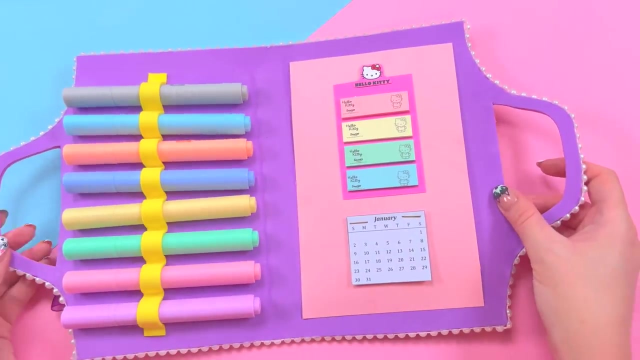 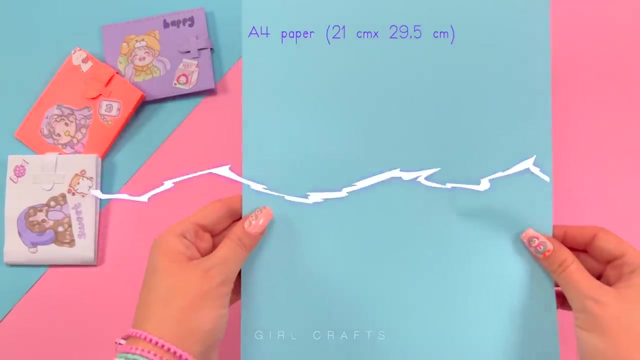 Hello, sweetheart, isn't it a sunny day? time to throw your cares away and kiss me. Let's go climbing up into an apple tree, See what all the birdies see and hear them sing. When love's in the air, I put dandelions up in my hair. 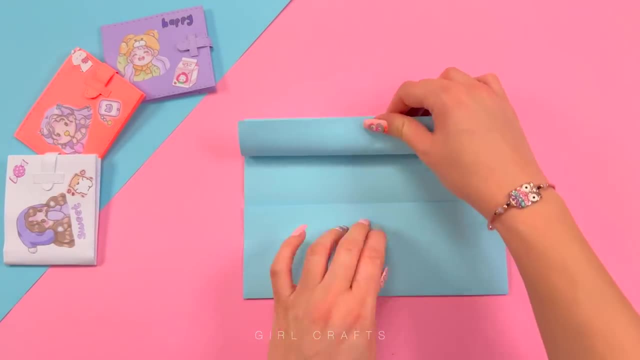 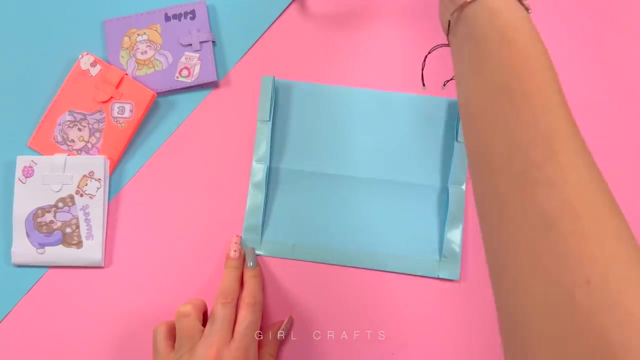 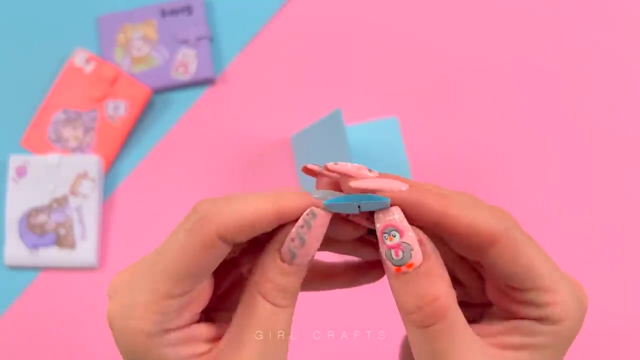 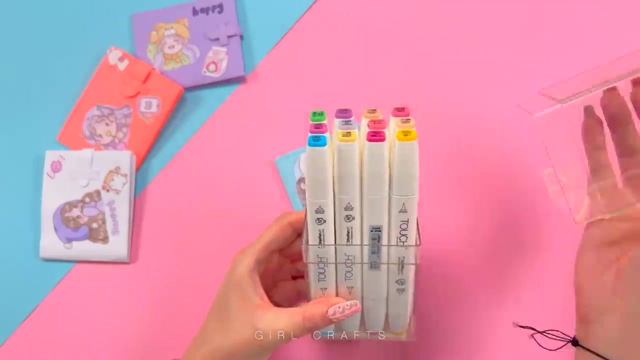 Cause you make me feel like I am free Boy. you are sweet, my God it be. Hello, sweetheart, isn't it a lovely night? The moon is shining oh so bright above us. Angels sing. whenever you sit next to me, I feel a glow come over me like heaven. 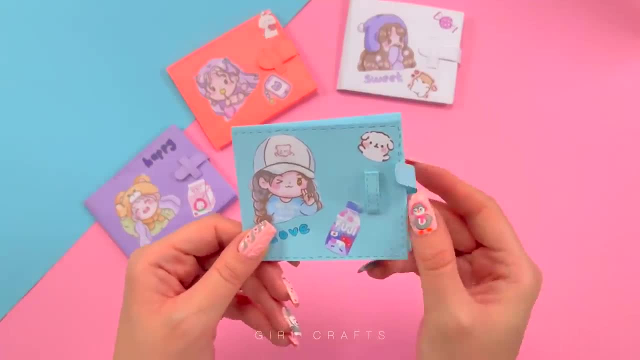 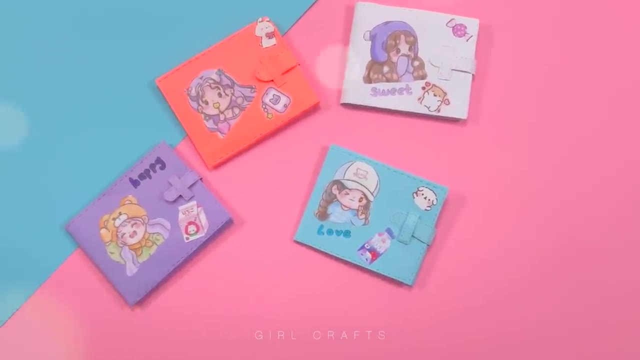 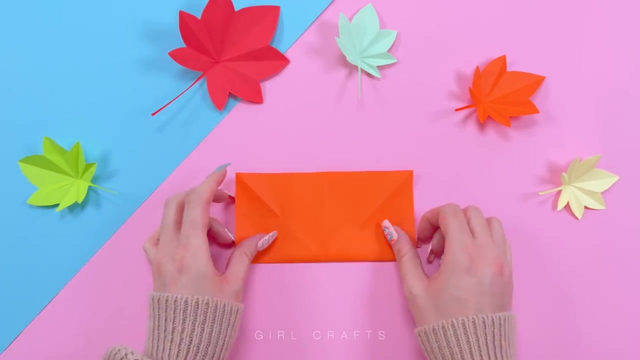